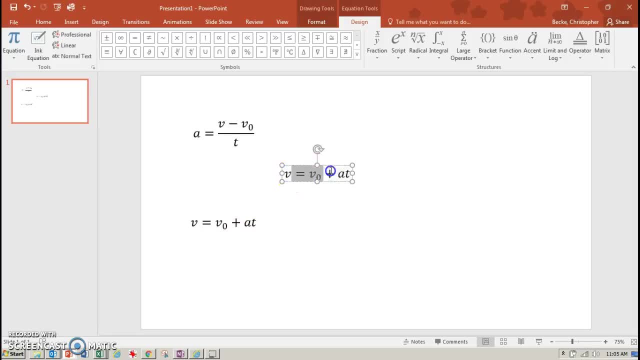 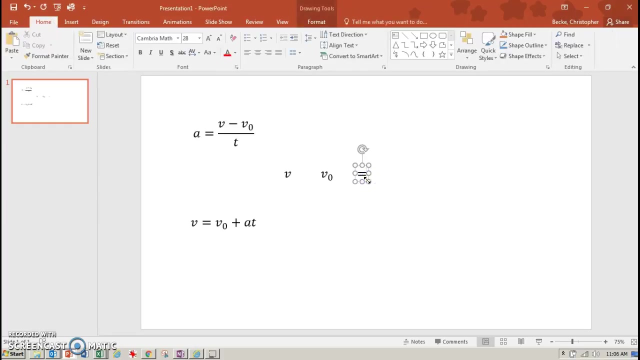 duplicate that. If I take this and I say: this is my v, so this is just a v, Let me duplicate that and this is going to be my v0. So let me make that my v0.. So what I'm doing is I'm making each individual point of each individual part of my old one become a new one. So let me get rid of that and make that an equals. Let me make the next one a, a and a t. So duplicate that for a and duplicate that for a t. So there's my t and this one will be my a, and then I should be mostly there. So I'm going to duplicate that. 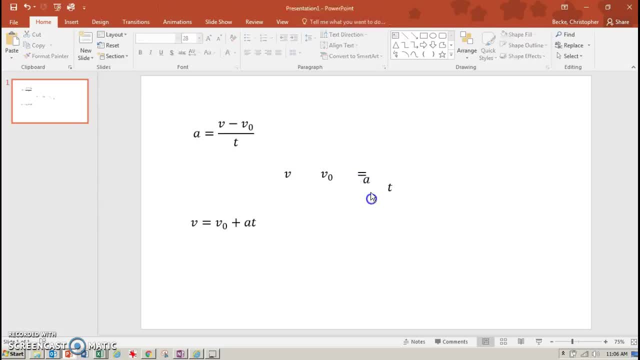 So sorry I had to sit through that. Hopefully you fast forwarded The next step. if I want to animate it, I want to take this a and kind of overlay it where that a was. I want to take this t and overlay it where that t was. I want to take this v and overlay it where that v was. I'm going to need a minus. I have my equals, So I put my equals where my equals goes And then I have my v0. 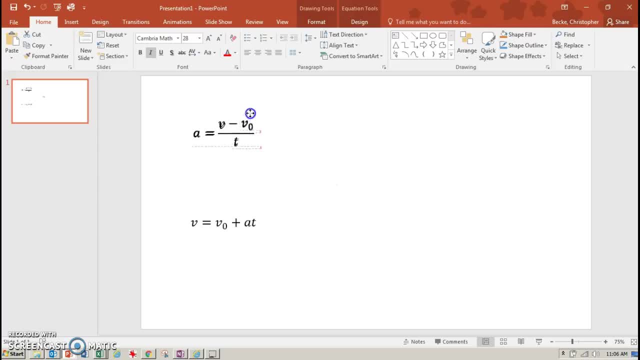 Which I can move to where I put my v0. And then I'm going to need a minus. Actually, the minus is going to become a plus, but yeah, we'll do that anyway. So this is now a minus, So the minus goes where the minus goes. Now that's a big mess. So, to get it precise, let me zoom in, And I usually hold down alt, And that way I can kind of take a look at where they are. You can't align because you're not aligning. 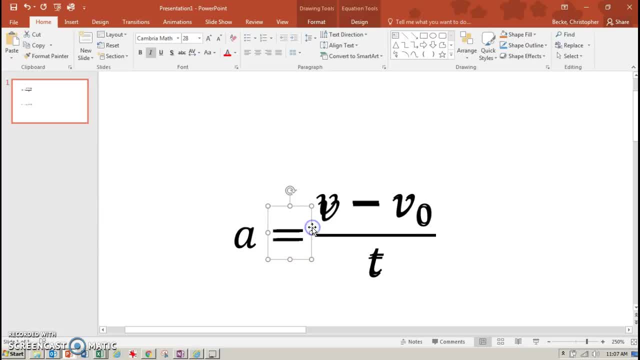 So I'm actually using the center of an object or the side of an object. So if you want to fast forward to this as well, you can. Once I have my objects aligned pretty good, then I'm going to add motion paths to them, And it's a pretty simple motion path. It's just a down, But again I want to align it with something. So there's my t. 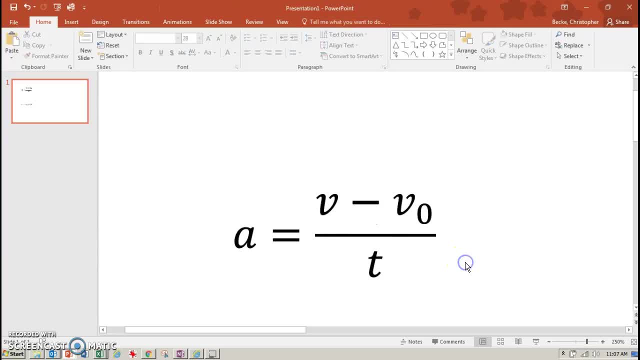 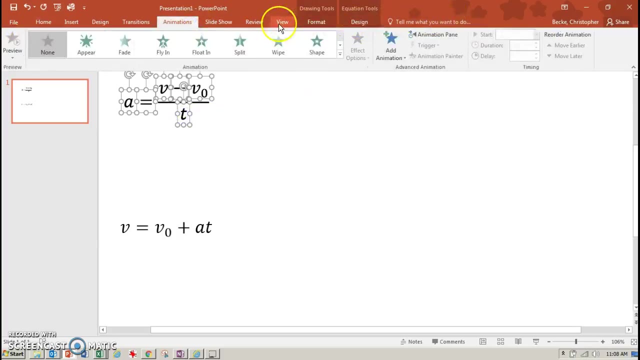 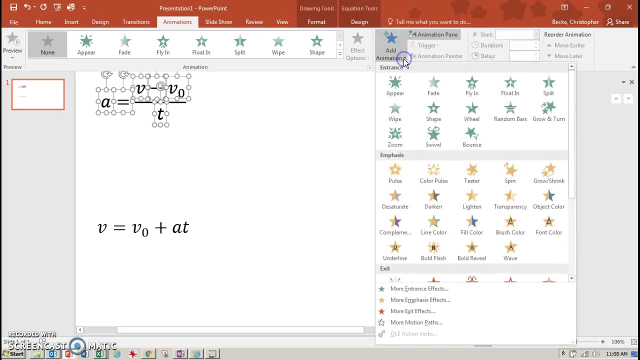 So now I've got my t. So now I've got my t And I've got the overlaid variables that I'm going to move. So let me zoom out just a little bit. Now I want to move motion from a and the equals and the v and the minus and the v0 and the t. And now if I look at my animations and I show my animation pane, There's my animation pane. What I want to do is I want to add an animation And I don't want an entrance, I don't want an emphasis, What I want is to add action. 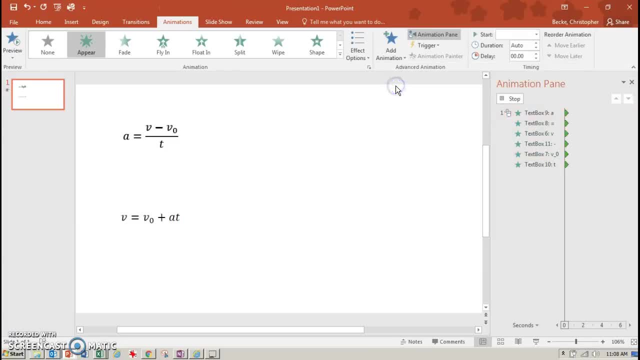 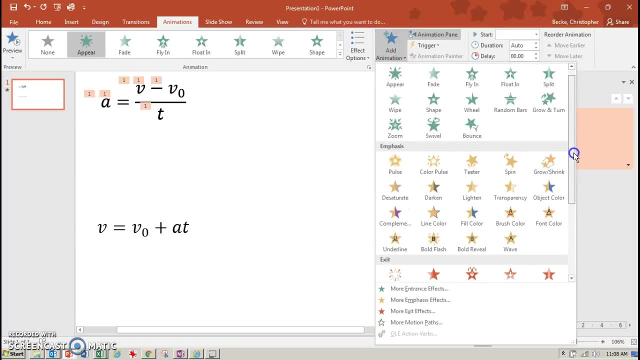 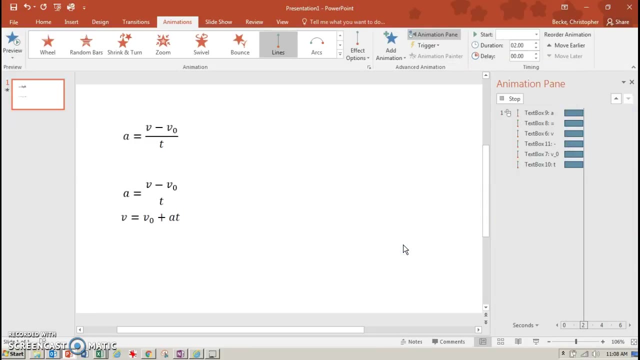 Actually, let me do that. first, I'm going to add an appear on all of them, So they're going to pop out on top. That'll make it if I'm slightly off, it won't be sitting there too long and looking fuzzy. Now I'm going to go down here and I'm just going to add a motion path line. I just want everything to move down, So when I click on it it's going to move down. So now I have two types of animations: I have my appear and I have my motion. Now what I can do is I can zoom in a little bit on where I want them to end up. 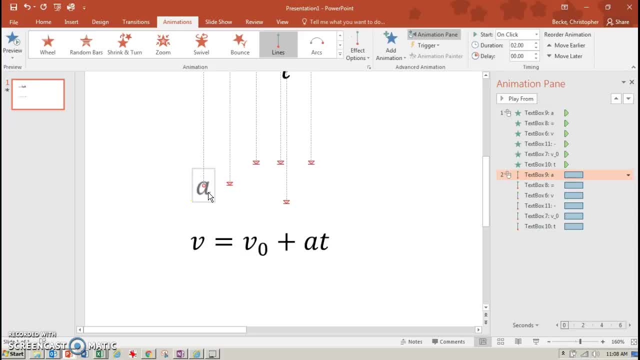 So here is: if I click on this red, that's where the a will wind up. Well, I want my a to wind up over here. In order to fine tune it, I can hold alt. This next red arrow is my equals, So I can hold on that and hold my alt key to fine tune where I'm placing it. I can take this one and that's going to be my v. Well, my v is going to wind up over here. My next one is going to be my minus. My minus is actually going to wind up here and become a plus. 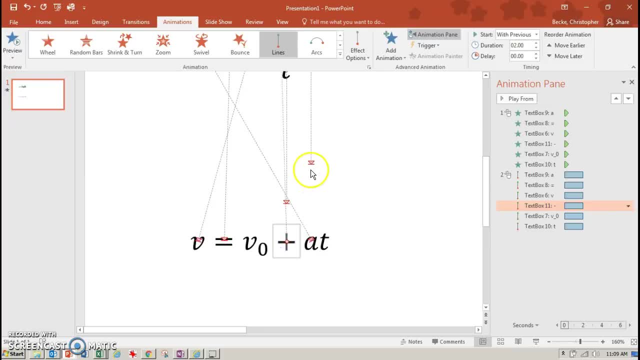 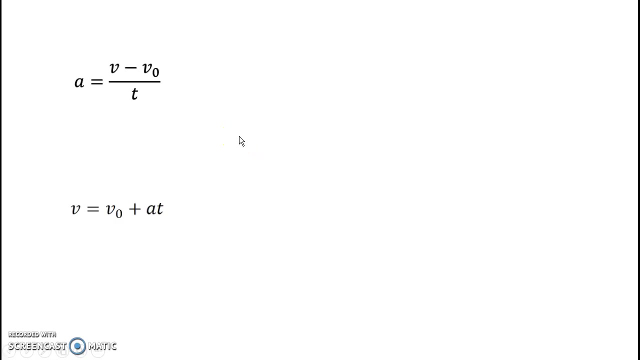 But still I want to move it to the right place And I'm going to take this one and that's my v0.. Let me move my v0 over here And finally I'm going to take my t and move my t over here. Now I could get really careful and see where they wind up. Now, if I preview that, you'll see that I start with my equation here. As I click, then my variables appear. As I click again, my variables all move to the right place.